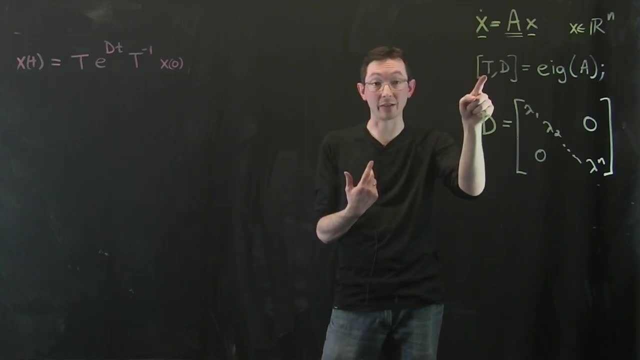 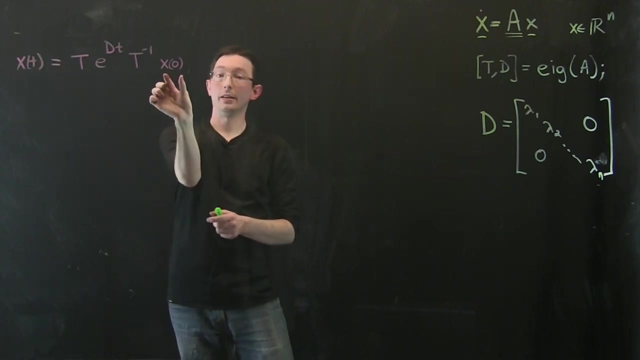 So in MATLAB, very, very simple to get a matrix of eigenvectors t and a diagonal matrix d that has only the eigenvalues- This should be lambda n, Only the eigenvalues, Only the eigenvalues on the diagonal, and zeros everywhere else. And then, in terms of this matrix of eigenvectors and eigenvalues, it's easy to solve the system x at some later time. t in terms of the initial condition and these relatively easy to compute matrices. 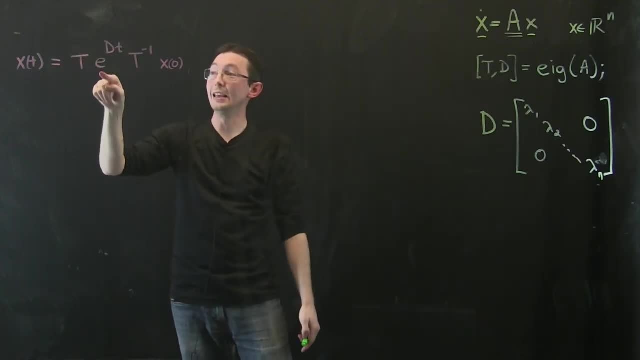 t again, matrix of eigenvectors: e to the diagonal d times time, which is easier to compute because it's diagonal, and t inverse. Okay, and so what we're going to talk about next is the matrix of eigenvectors. 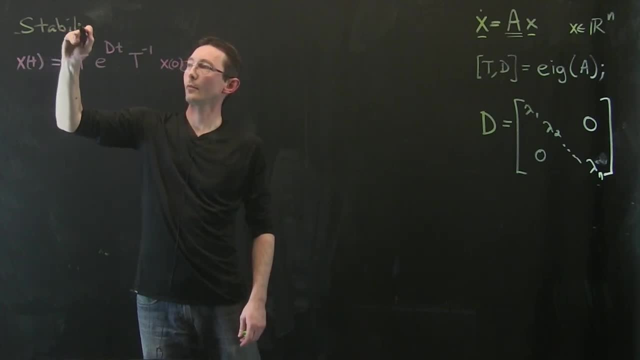 And what we're going to talk about now is essentially stability. Okay, so we're going to talk about the stability of the system, which basically means: what does the system do as time goes to infinity? Does it blow up? Does it all go to zero? Does something weird happen? 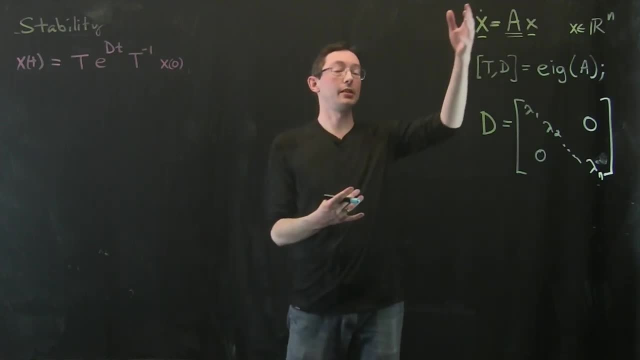 Okay, now there's whole classes on ordinary differential equations and linear algebra and dynamical systems And we'll talk about phase portraits and saddles and syncs and centers and all kinds of deep and very interesting stuff. But we're just going to talk about it later. 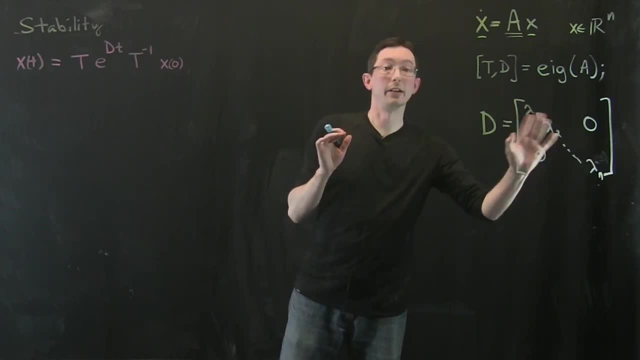 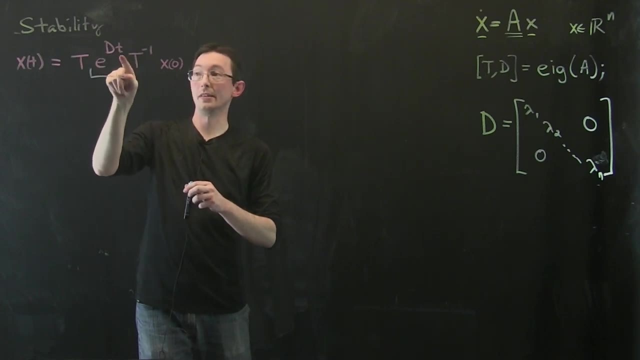 All right, so let's get started to get kind of the bare minimum that you need to understand. stability here, okay, And it all has to do with this. e to the diagonal matrix, d times time. So this is where things happen as time goes to infinity or in this term, And what's nice. 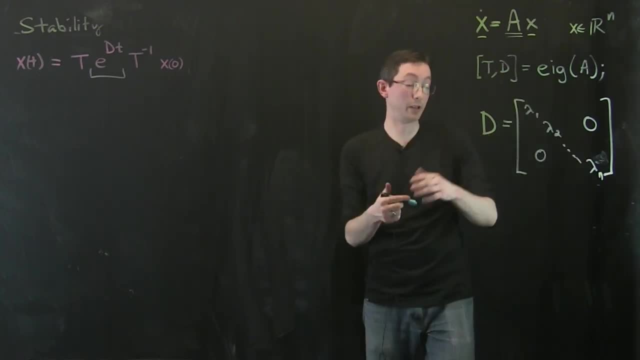 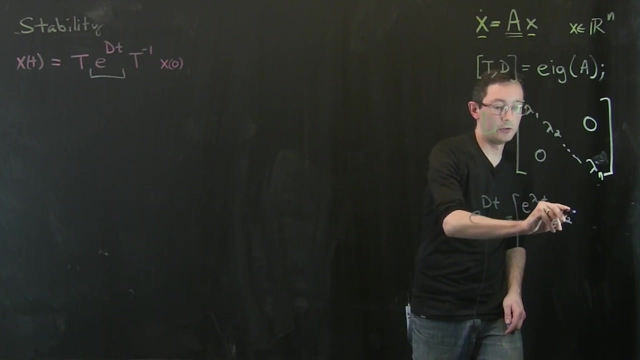 about diagonal matrix of eigenvalues d- and this is just a rehash of last time- is that e to the diagonal? t is easy to write. okay, It's just e to the lambda 1 time, e to the lambda 2 time, dot, dot, dot. e to the lambda n time on the diagonals. 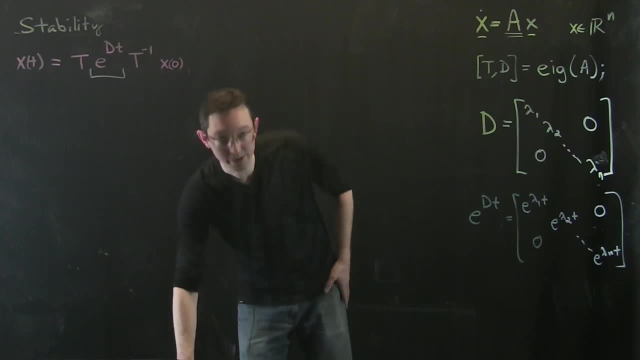 and 0 everywhere else okay, And so basically what we're going to find is that if any of these matrix exponentials blow up to infinity, then this whole mixture- so I think, of these eigenvectors t and t inverse, is almost like taking 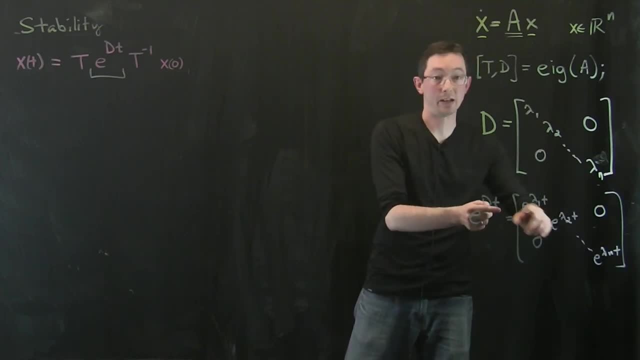 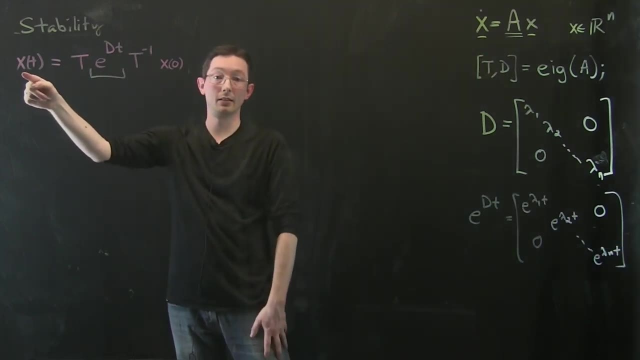 some mixture of these different basic frequencies that we're going to find. And so what we're going to find is that if any of these are time dynamics, these each e to the lambda 1, lambda 2, lambda n dynamics, and you're mixing them up to get what the dynamics are of your original state x. 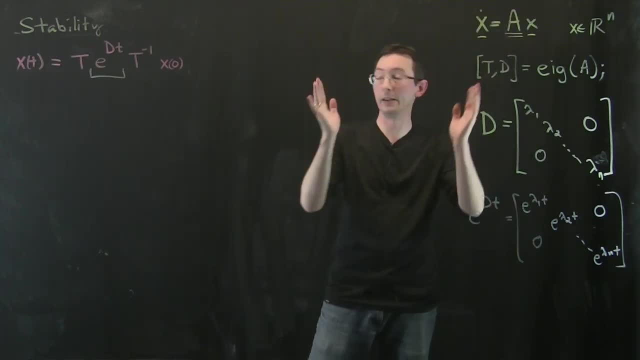 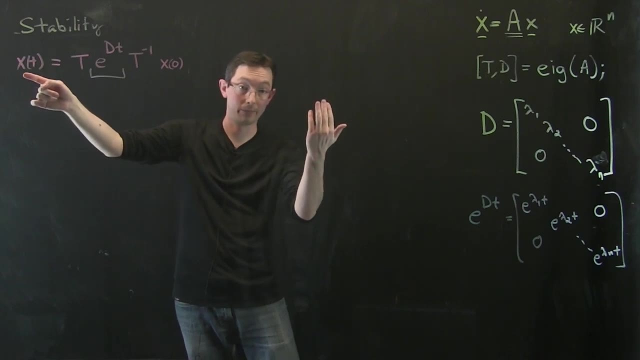 okay. And so if even one of these blows up to infinity, then essentially, if you add that into the mix, then x is also going to more or less blow up to infinity. okay, Especially if you take some random initial condition that has some component in all of these eigenvector. 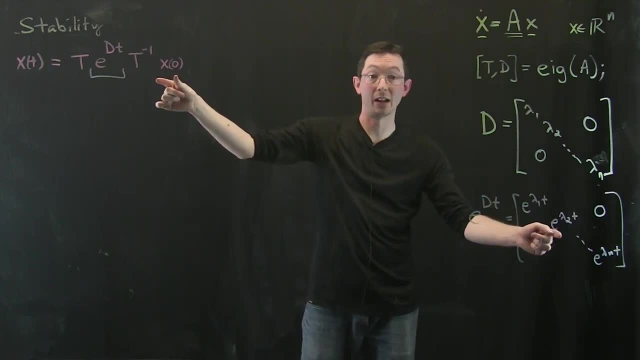 directions, then chances are it'll have some component in an unstated eigenvector direction and that will blow up to infinity, okay. And so what do I mean when I say blow up to infinity? Well, each of these eigenvalues has a real and an 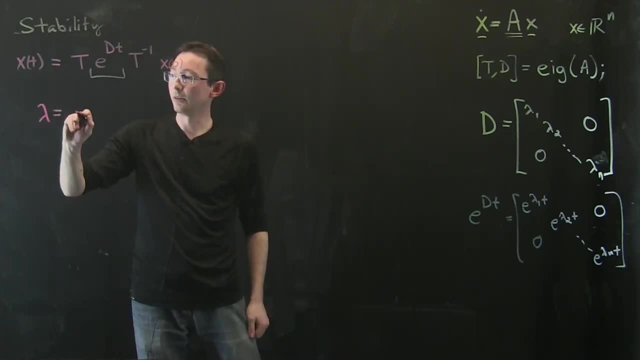 imaginary part. So let's say lambda equals a plus i b, and this is just kind of going through complex analysis. So if I take e to the lambda t, then that equals- what I'm going to write down is just Euler's formula. so it's going to equal e to the a t. that's a real valued. 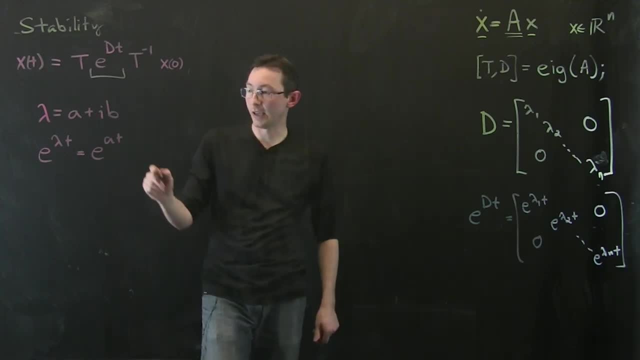 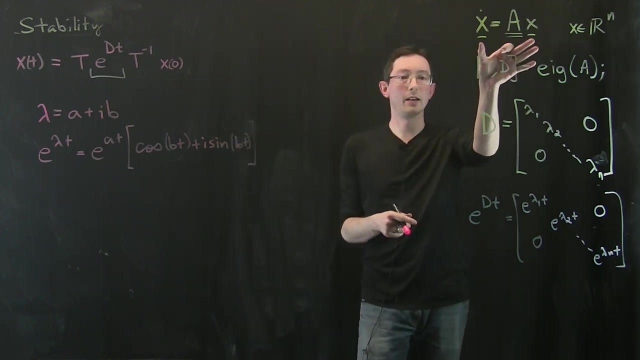 function of two real scalar arguments: a and t times cosine of bt plus i times sine of bt. okay, Now it's a little weird in a real valued system. so like: let's say: all of x are real, they're real and all of the coefficients of a are real. 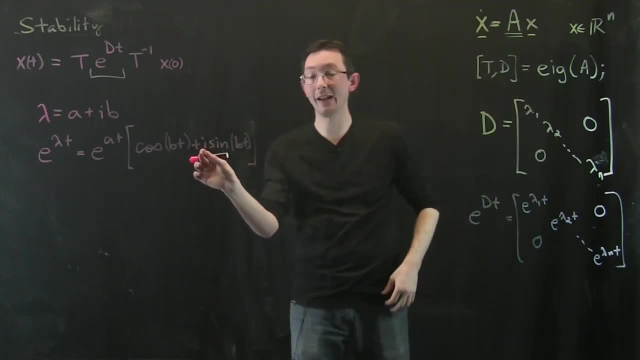 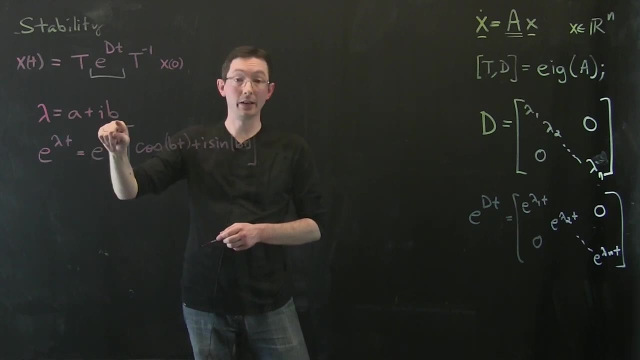 then this should be real forever. So why am I getting an imaginary here? That's a little weird. Basically it's because if I ever had an eigenvalue with an imaginary part for a real valued system, it would always come in a plus or minus pair. so 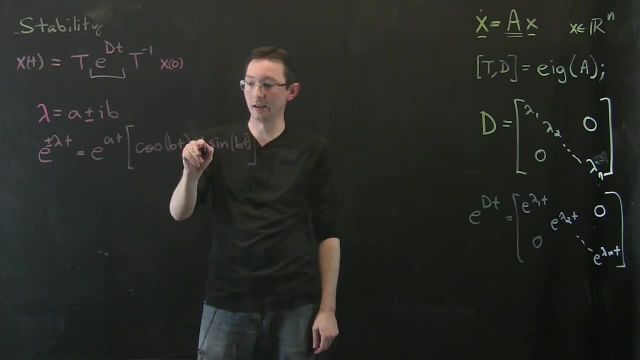 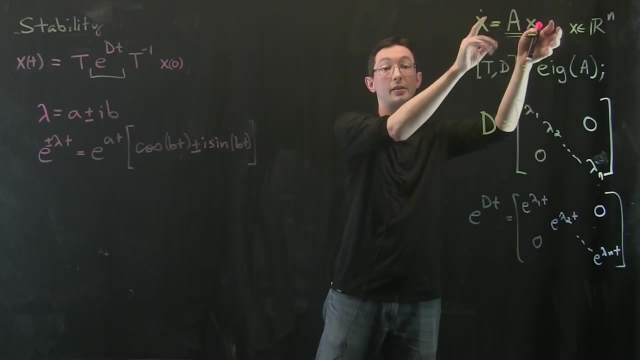 that I would have this plus or minus lambda t and I would get a plus or minus i sine bt And basically the physics or the math of the situation would be so that the solution, when you take that mixture and add it to the solution, when you add them up, the imaginary parts cancel and you just get. 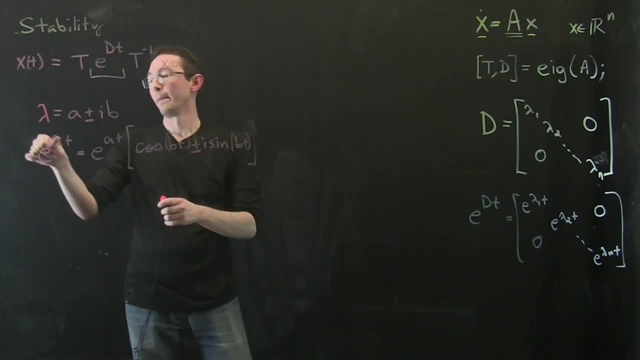 real valued outputs, Again a little deeper. but all I want you to know is that, essentially, if I have a complex eigenvalue- a plus i b, this is how it breaks up. Now notice that cos plus i sine, this never has an amplitude larger. 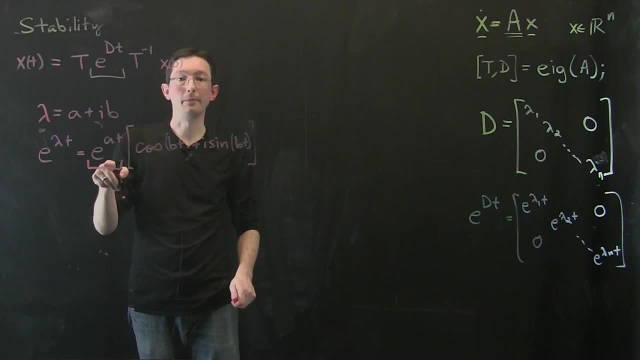 than one. it's always equal to one, and so this tells me if my solution is growing in time or not. We're decaying in time, okay, And so if a is greater than zero, then essentially what that means is that I have this exponentially growing envelope. Maybe my 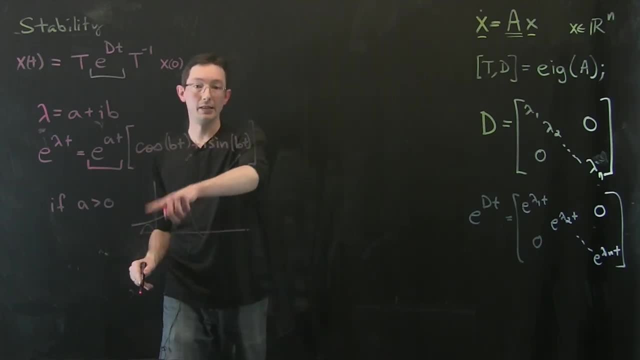 system is oscillating sinusoidally, but it's doing so in this exponentially growing envelope and it'll eventually blow up to infinity. And if a is less than zero, then I have an exponentially decaying envelope, and so my system is going to decay to zero as time goes to infinity. 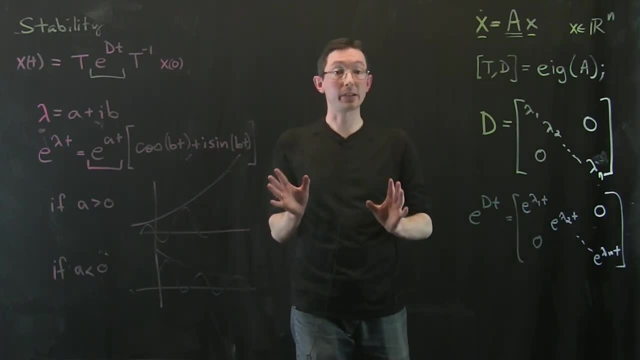 So this is really simple to understand. If all of my eigenvalues d in d, if all of these lambdas in d have negative real part, if all of the real parts, the a's of all of these eigenvalues, are negative- the real part is negative- then all of my 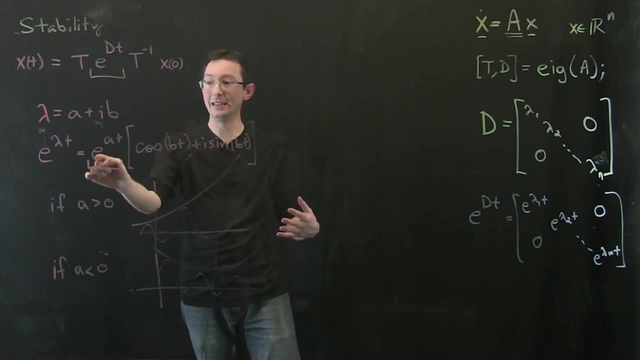 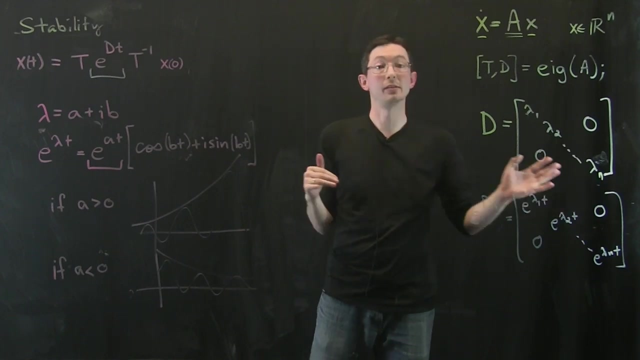 dynamics are stable. All of them are multiplied by e to the negative number t, which gets closer and closer to zero as t goes to infinity. And so this system is stable if, and only if, all of the real parts of all of these eigenvalues are purely negative, If even one of these eigenvalues has a real part. 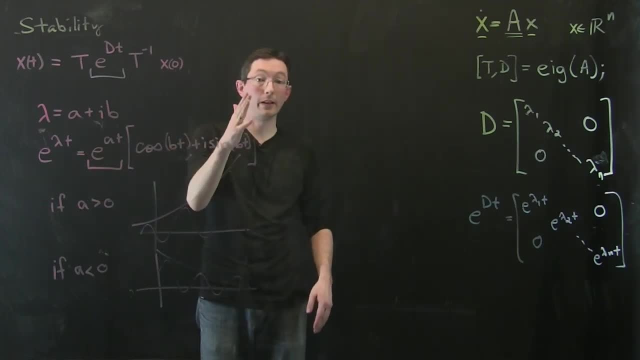 that's positive, then that component will blow up to infinity and it'll cause my state x to also blow up as t goes to infinity. Okay, So it's really simple to say and it's also pretty simple to write down, And so what I like to do is, I think, 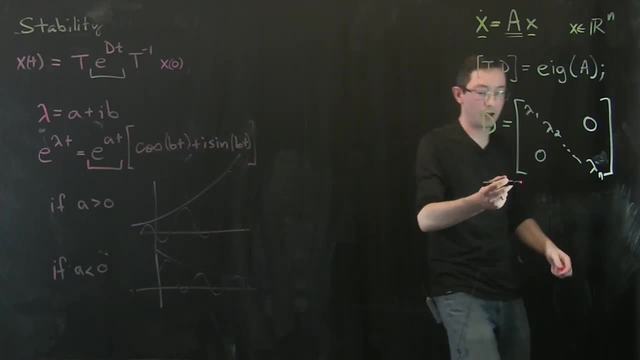 about these eigenvectors, sorry eigenvalues, as living in the complex plane, And so if I say lambda is in the complex plane, it is stable. everywhere here where the real part is negative, Everywhere in the left half plane, this is where a is negative. The real part- remember this- is real. sorry, this is. 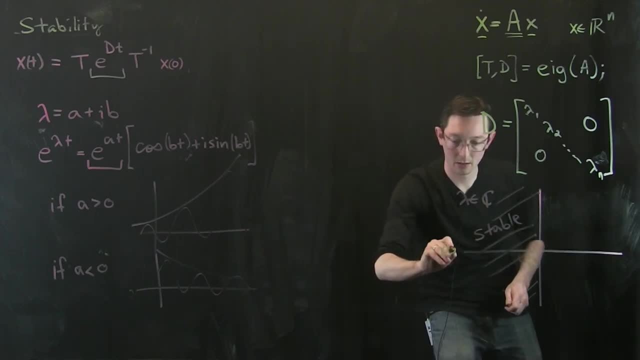 failing. This is real and this is imaginary. So anywhere that the real part of lambda- the a part- is negative, it's stable, And anywhere where the real part is positive, it's unstable. And this is really simple to remember. is that, if any, 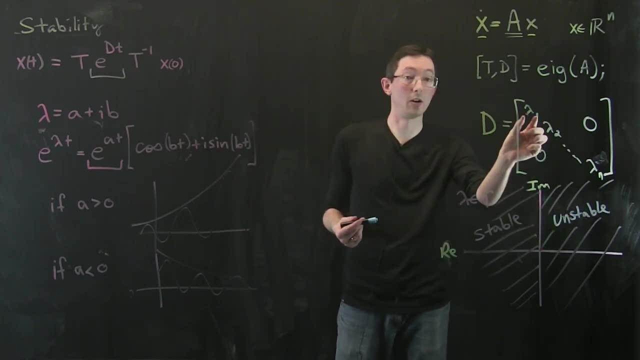 of your eigenvalues have real part that's positive, it's unstable. If they all have real part that's negative, it's stable. And so a big part of what we're going to do in control systems is we're going to start with an A matrix where maybe we 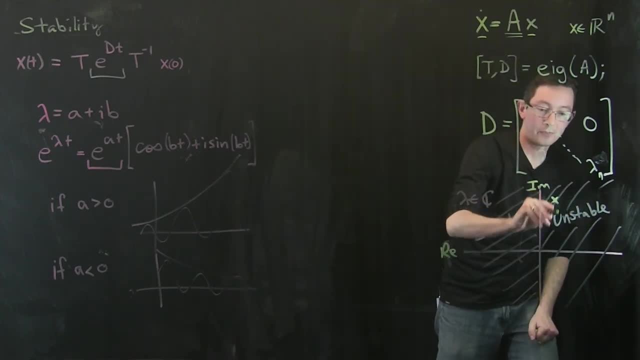 actually have some unstable dynamics. Maybe we have a couple of eigenvalues out here that are a little bit unstable And by adding plus bu we're going to try to drive the system into stability. We're going to try to force those eigenvalues. 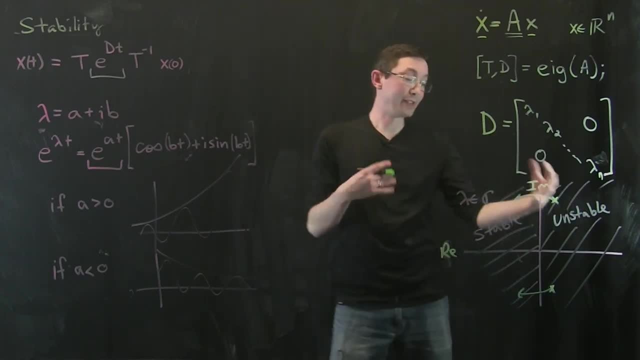 to become stable again, Okay. so this is really cool and this is a nice picture that allows you to think about what we want the system of A to look like, So we can characterize what we want to do, And so what we're going to do is we're going. 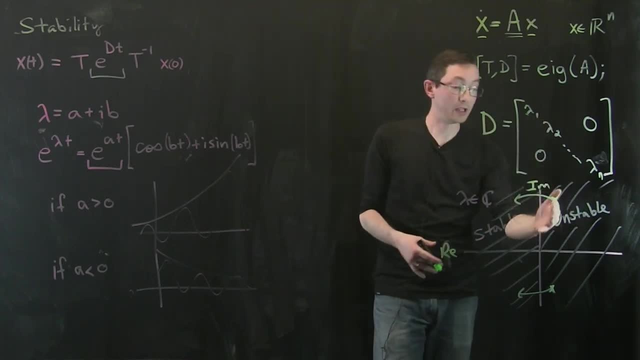 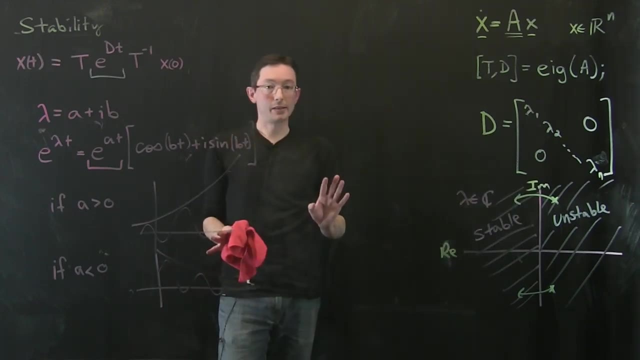 to try to make this system of A to look like almost entirely based on its eigenvalues, because we want to drive them into the stable left half-plane in the complex plane. Okay, Okay, makes sense. so far We have a dynamical system. The solution depends on the eigenvalues. 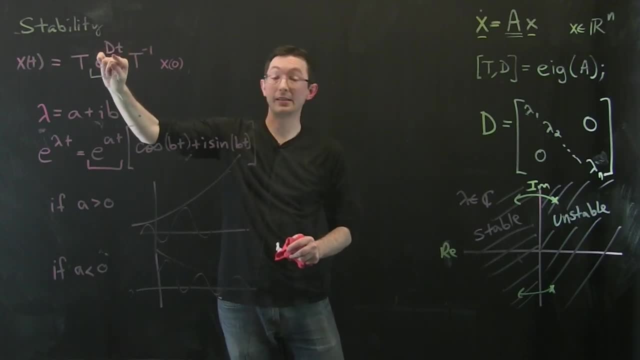 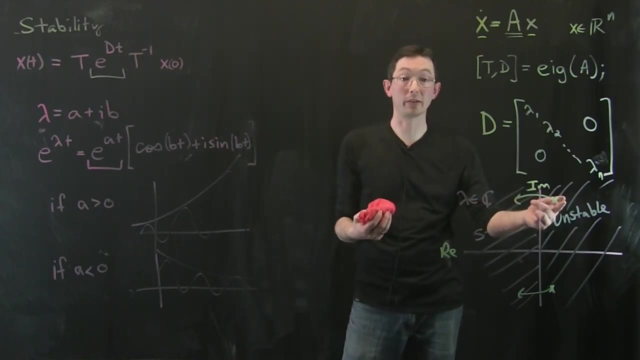 and eigenvectors, but its dynamics in time only depends on the eigenvalues in this diagonal matrix D. If those eigenvalues- and they can be complex, if they have a real part, that's positive. any of them, the system is unstable and it blows up. So the inverted 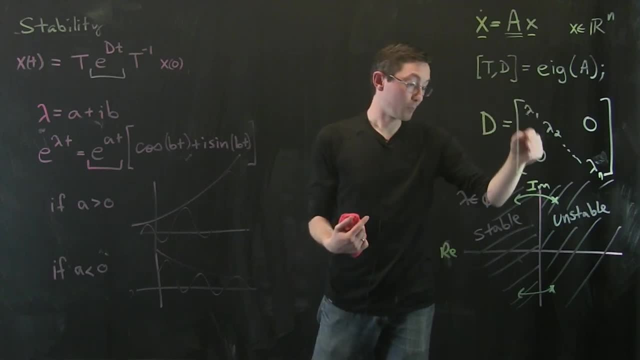 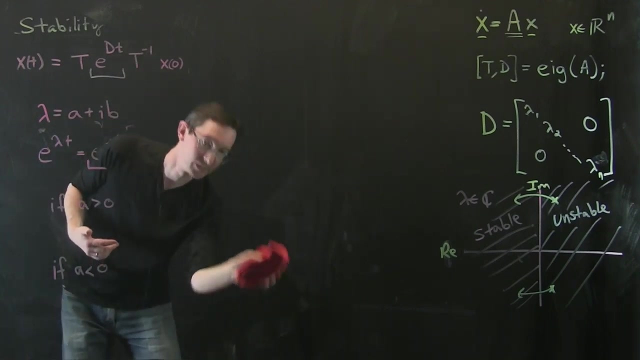 pendulum has an eigenvalue with a positive real part, and that's why it's unstable and it starts to blow up. Okay, so that's pretty intuitive, and I think, again, most of us have that intuition about stability and eigenvalues, and so the next thing I want to do is get into discrete time systems. so this is a 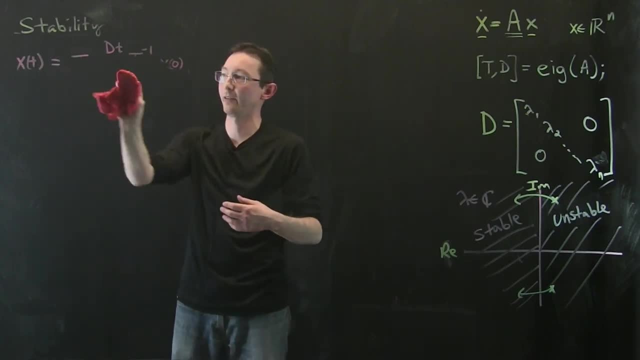 little bit less common to a lot of you who have an applied math background or a background in ODEs and linear algebra, but in control theory this is really bread-and-butter stuff. In physics we write down systems: x, dot equals ax or x. 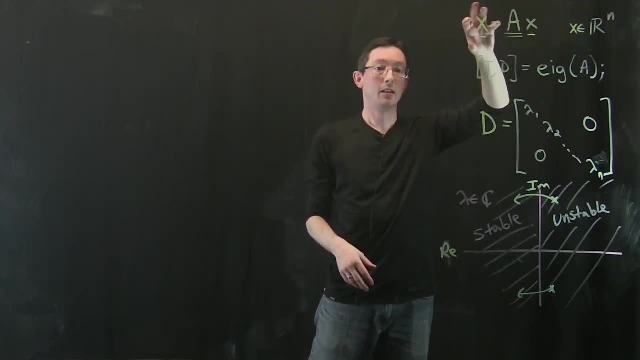 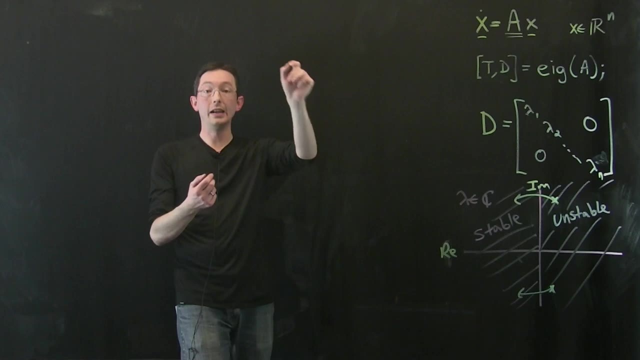 dot equals f of x in terms of this continuously varying function x of t. but in a physical system, if I have an experiment or if I am recording data from a system, I don't have a continuous measurement x of t. What I do is I: 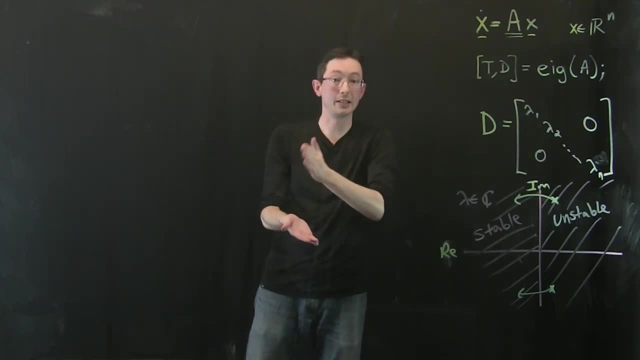 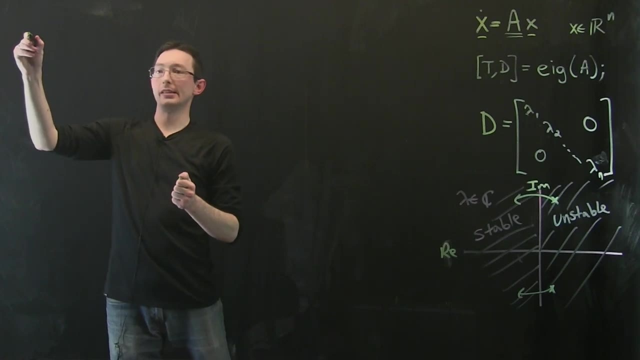 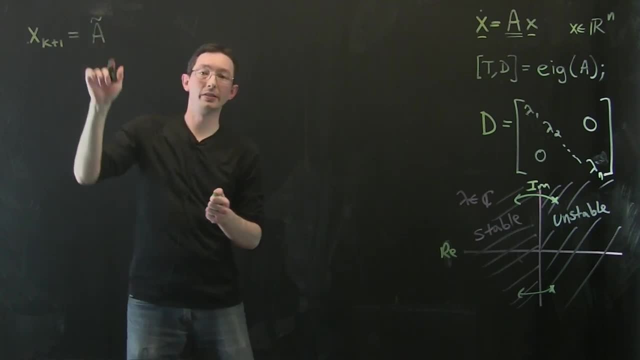 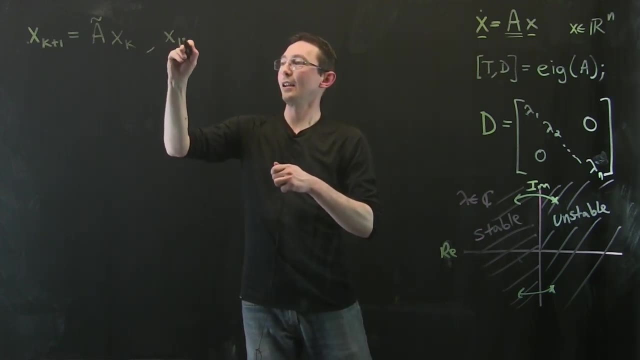 equals some new matrix. I'm going to call it a tilde times x, at the previous time k. And let's be super explicit here: x of k equals this continuous x evaluated at k delta-t. okay, So I take some system. it might have an underlying continuous dynamics. 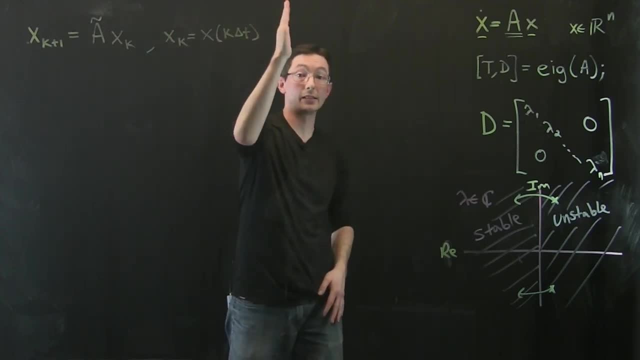 but I'm going to measure it at these individual delta-t instances of time and there's some discrete update that tells me if the state was x at time k, here's what the state's going to be at the next delta-t at time k plus 1, okay. 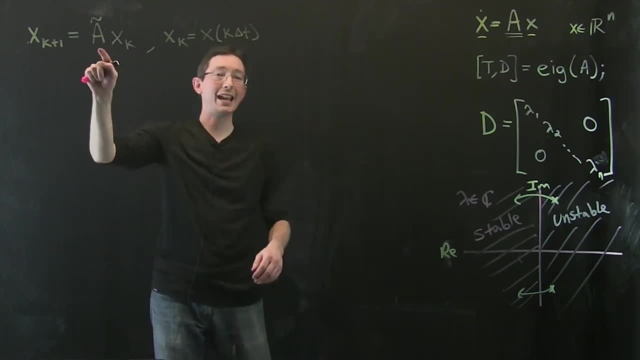 And it's also nice just to write down what this a tilde is in terms of a. so this is also super simple: a tilde, A tilde is just e to the, a delta-t, okay, And we spend a lot of time just now deriving that. 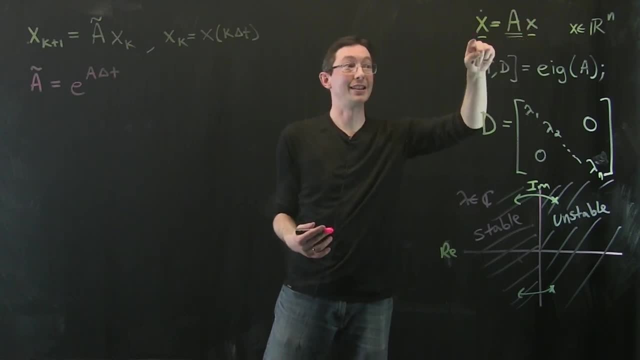 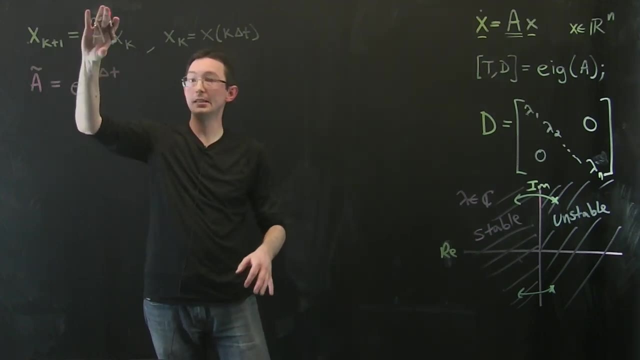 that if I had some dynamics and I wanted to figure out what it is at the next you know plus delta-t in the future, all I have to do is map it by e to the a delta-t. okay, So these two matrices are related intimately by the matrix exponential, okay. 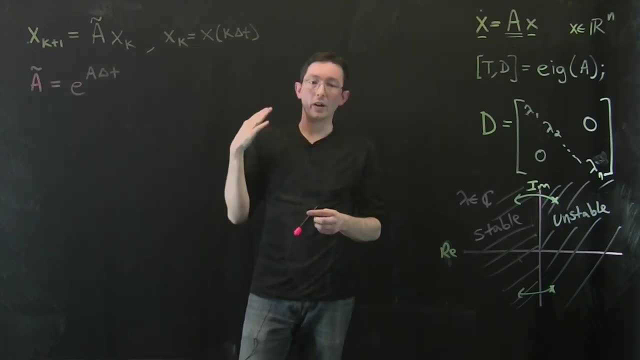 But we're not going to use that so much here. What's really interesting is we have a notion of stability in continuous, continuous time, so having to do with the real part of the eigenvalue. In discrete time there's also a notion of stability. 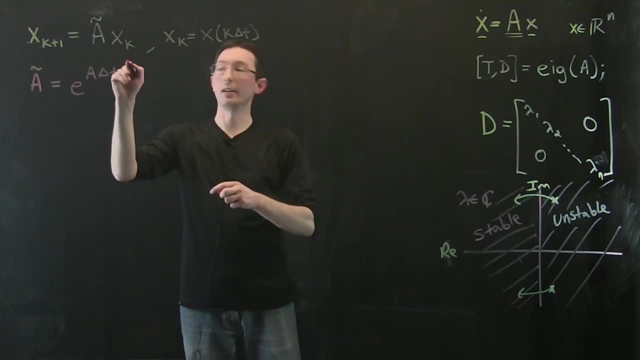 but it's a little bit different, And so that's what I want to walk you through right now. okay, And I'm just going to kind of cordon this off, So the notion of stability that I want us to talk about now. 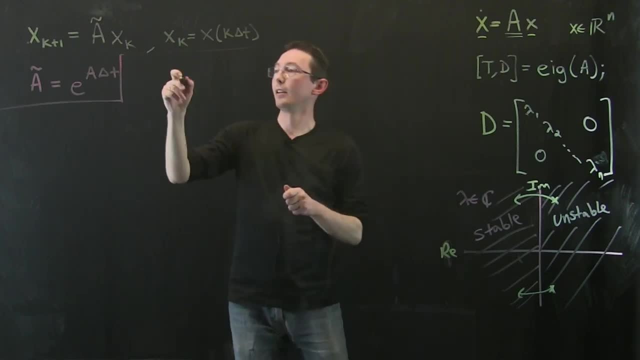 let's say that I have some initial condition. I'm going to say I have x naught. okay, Given that initial condition, I can compute the whole trajectory or the whole set of measurements for all future times just by multiplying by a tilde. okay, 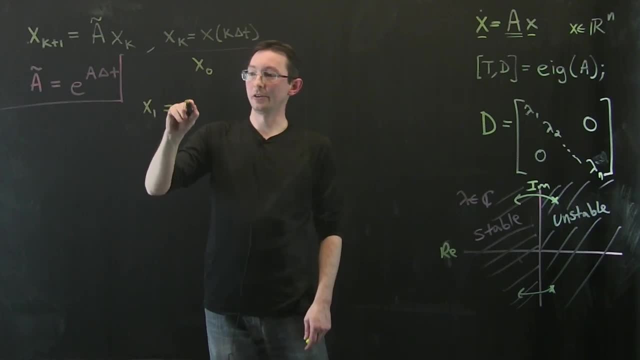 So if I have x naught, then x1 is just a tilde times x naught, right? That's exactly what this says: x naught. So if I want x1, it equals a tilde x naught. If I want x2, it's equal to a tilde x1, which is a tilde squared x naught, okay. 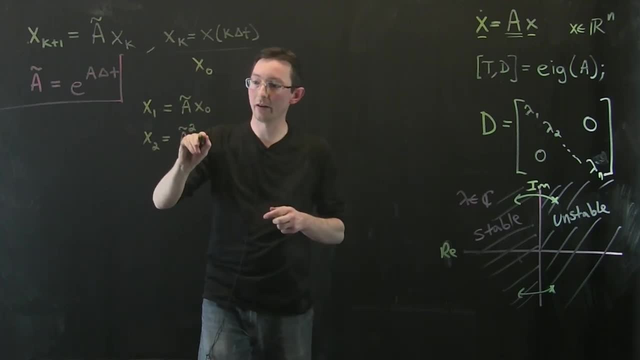 So x2 equals a tilde squared x naught. I'm going to say that one more time: x2 is just a times x1, or a tilde times x1, which is a times a times x naught. So x2 is a tilde squared of x naught. 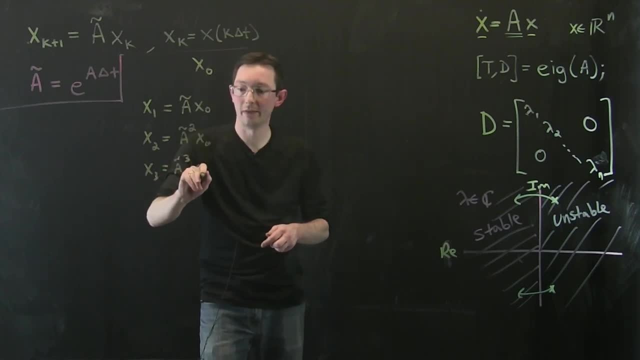 x3 is a tilde cubed of x, naught and so on and so forth. So x at any future time. n is a tilde to the nth power times. my initial condition: x naught. Super simple, pretty useful. And what's really cool is I can take this exact same eigenvector and eigenvalue relationship. 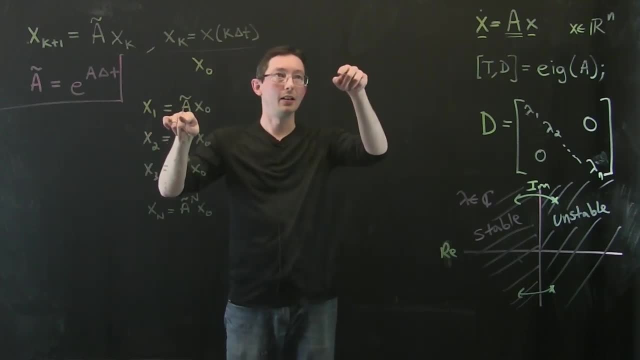 and I can say: well, a tilde is just- I forget if it's t inverse or t like t inverse dt. And a tilde squared is t inverse d squared t. And a tilde to the n is just t inverse d to the n t. 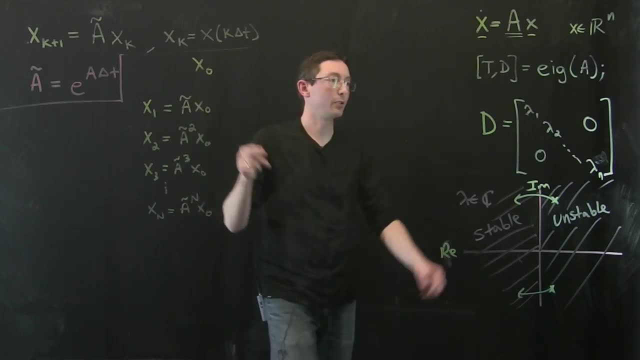 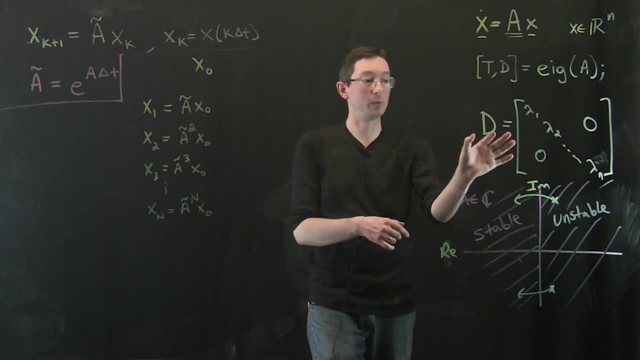 And so the only thing that really gets multiplied to all of these powers is this diagonal matrix. So in the continuous time case we saw that the only thing that got exponentiated was this matrix d. If I write this in eigenvalues and eigenvectors, the only power that increases again is this d. 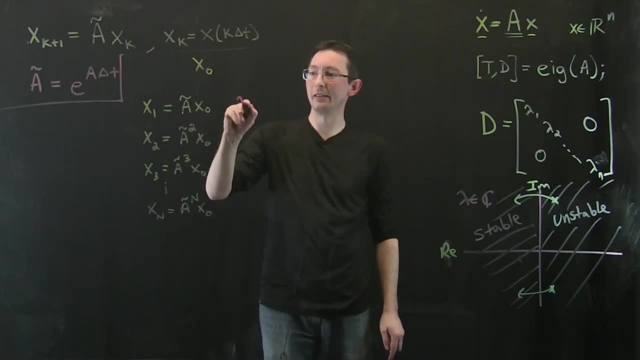 And so if we have some eigenvalue, let's say lambda, well here it's just, you know, lambda, here it would be lambda, squared lambda, cubed, lambda to the n. So if I follow what happens to an eigenvalue as I map it through this system, 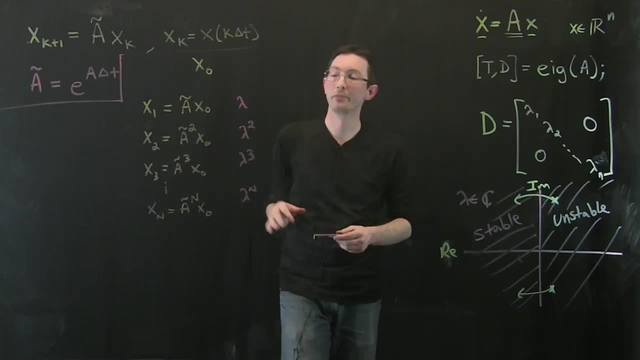 squared, cubed. fourth, you know all the way to the nth. what we find is that it's actually the radius of this eigenvalue that either grows or decays. Okay, so in the complex plane, what we have, I'm just going to draw a little complex plane here. 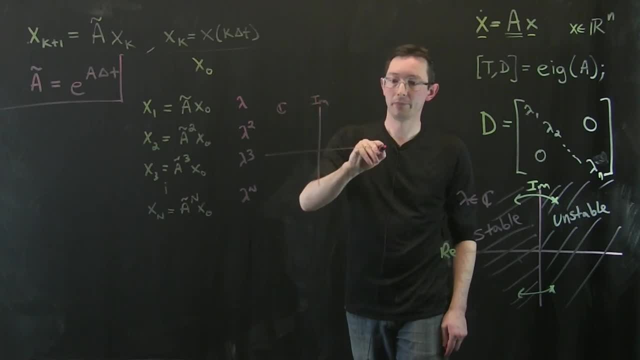 Complex plane. remember real and imaginary. Any eigenvalue lambda can be written as a radius and an angle theta, And I really love this representation. This is definitely how I always think about complex variables, almost always because I can say that lambda equals r? e to the i? theta. 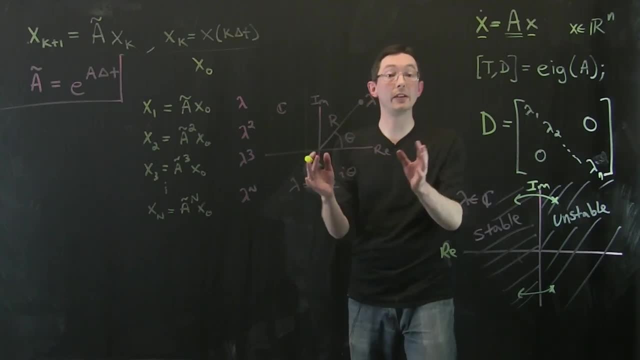 And when I think about things in terms of r? e to the i theta, and you can convince yourself, expand this out and you get cos theta plus i sine theta, and that's exactly what you get. The real part is r cos theta. 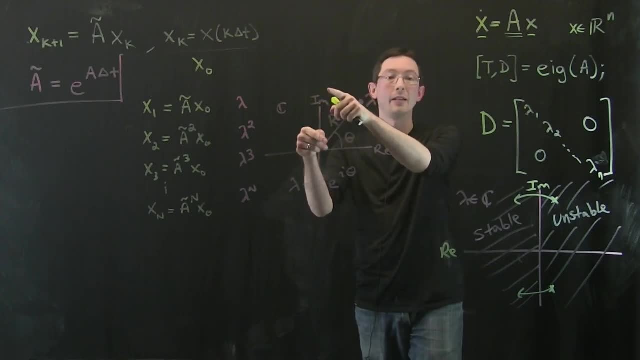 The imaginary part is r i sine theta or i times r sine theta. So this is true. But if I take lambda to the nth power and you can convince yourself, just multiply this out n times. it equals r to the n, e to the i n theta. 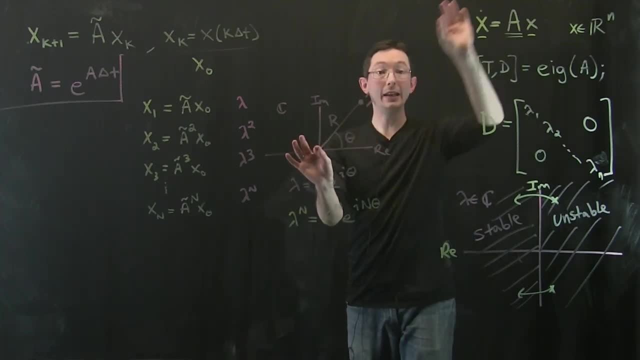 So what happens is the radius either gets bigger or smaller, but the angle just kind of rotates around and around and around. So if this radius is bigger than 1, this lambda to the n blows up as n goes to infinity, just like. 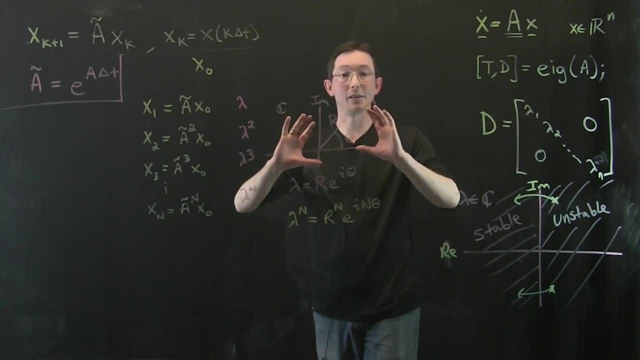 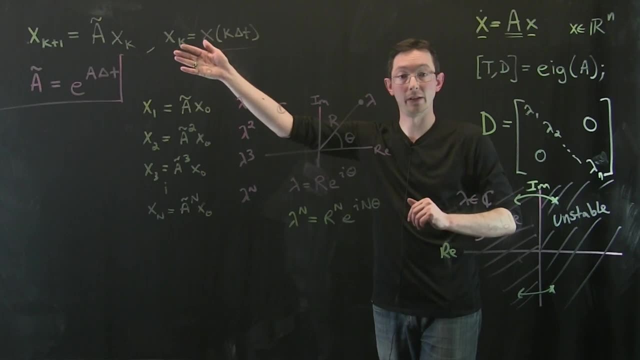 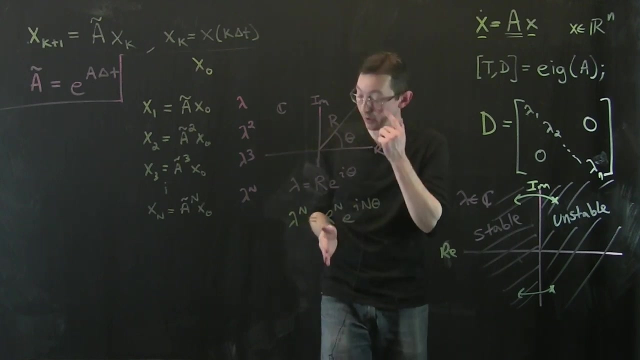 in the continuous time case, if this lambda has a radius that's bigger than 1, this will blow up as n goes to infinity, as time goes to infinity. And if the radius is smaller than 1, then this will decay to 0 as n goes to infinity. 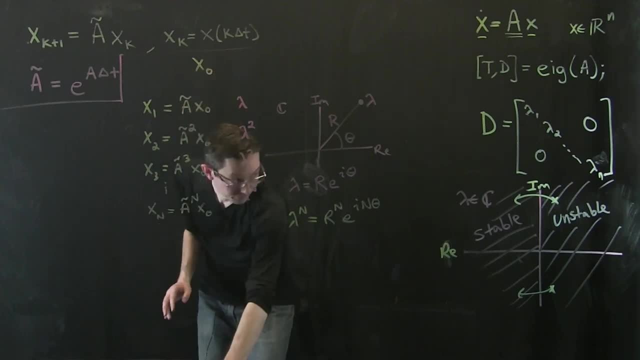 So now we have kind of a dual picture here. Again I'm going to draw this in the complex plane where all of my eigenvalues have to live. So now what I'm going to do is I'm going to draw some unit circle where everything inside has a radius less than 1.. 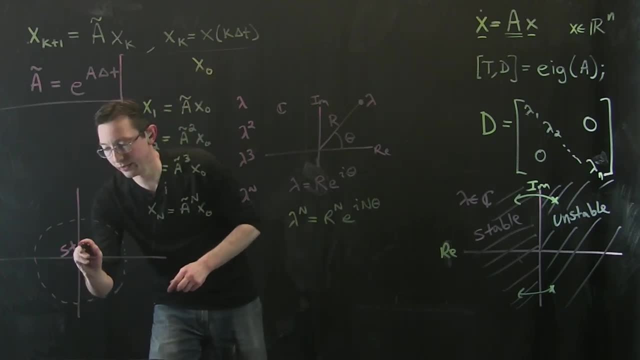 So this is my unit circle. Inside everything is stable in discrete time. So if my eigenvalues of a tilde live inside this unit circle where radius is less than 1,, this system is absolutely stable. And if my eigenvalues, if even one of my eigenvalues, has a real part that's bigger than 1,, 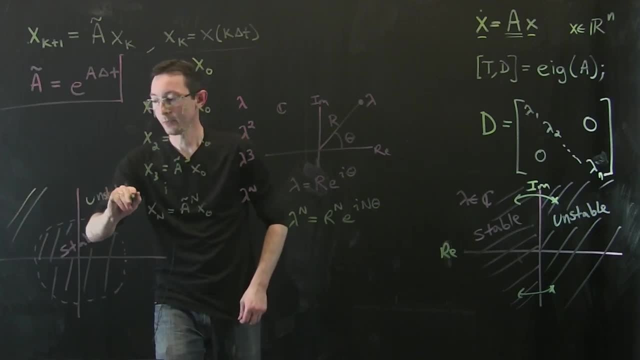 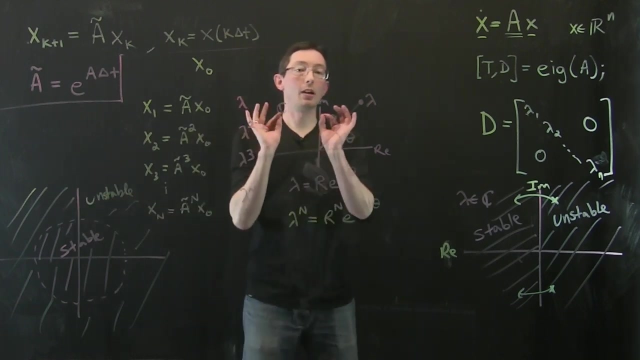 then everything out here is unstable. Okay, Because if I have even one of those eigenvalues with a real part bigger than 1, then this term blows up to infinity and this chain will blow up to infinity. Okay, And so I'm glossing over an important step. 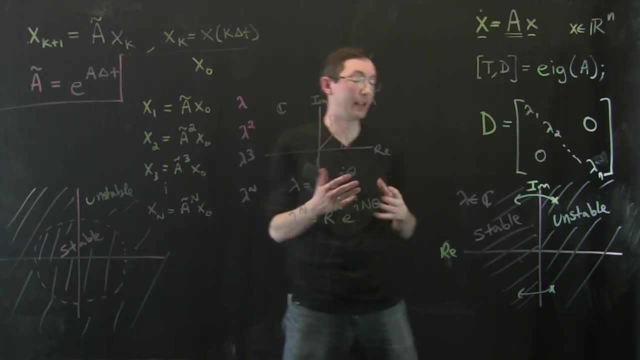 This is: if you're at home and you want to verify this and really kind of get expert at this, what you'll do is you'll take that expression and I'm just going to derive it because I can never remember it. I have. 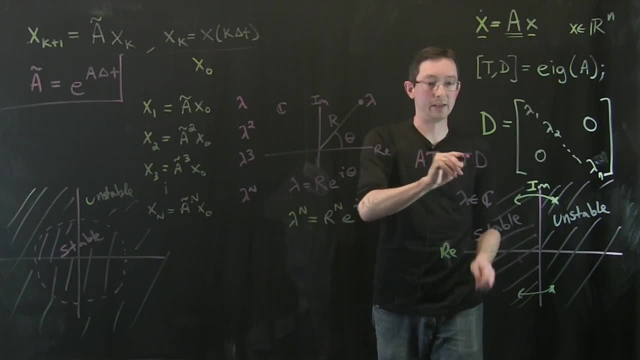 a time. t equals t times d. This is what I always start with. So a equals t d t inverse. I'm not sure if I said it right before And remember this is also true for a tilde- A tilde. 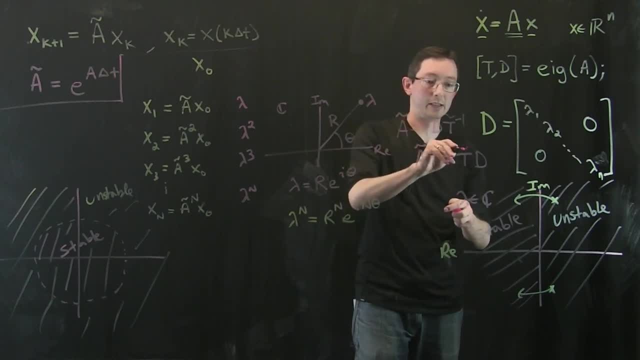 Okay, So that's also true, for, you know, put tildes on all these things. So I have some special eigenvectors of a tilde, some special eigenvalues of a tilde And what I want you to do to really convince yourself of all of this. 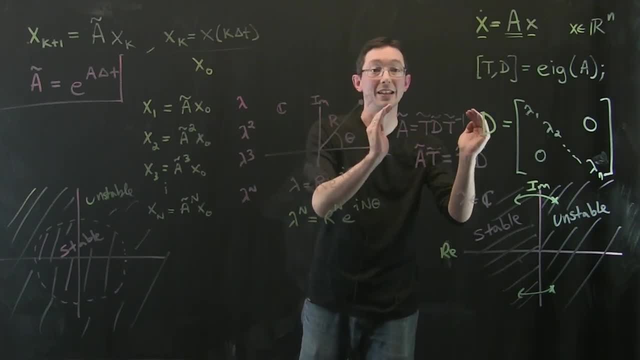 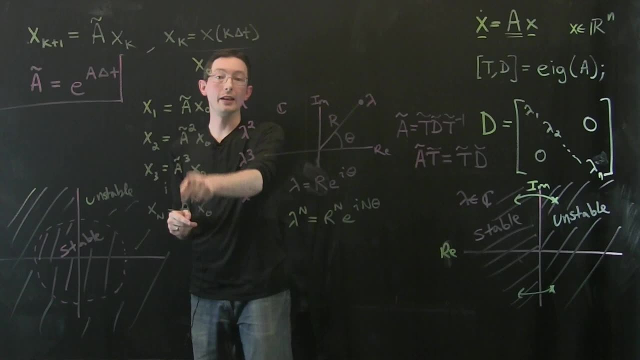 is: take this expression and I'm going to take this expression and I'm going to take this expression: a tilde equals t, d, t inverse- and plug it into all of these terms and you'll find that the only thing that could blow up or decay 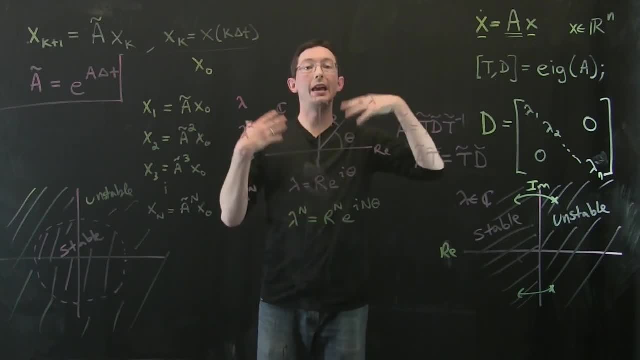 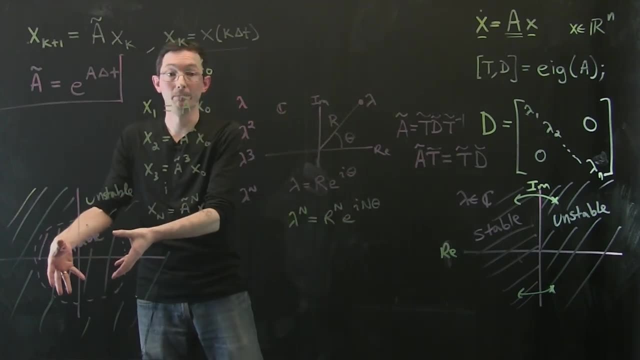 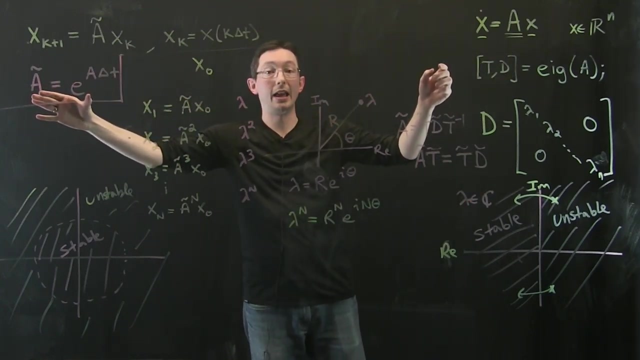 is this diagonal matrix d to the power n, And then you can convince yourself that all of the eigenvalues of a tilde have to be inside the unit circle for the system to be stable. Okay Now, and it's interesting because if you think of this matrix exponential that relates a tilde and a, 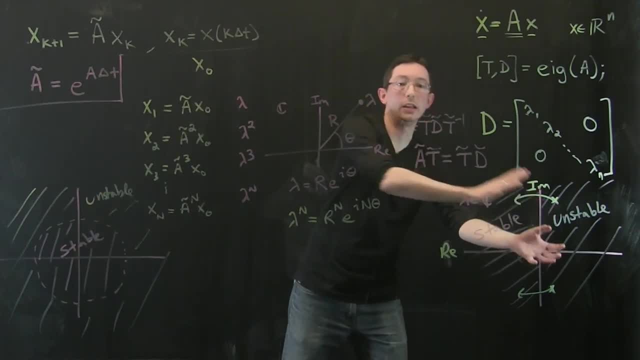 then that's actually a conformal map between these two complex planes, and this stable unit circle maps exactly to this left half plane under that map e to the a delta t. So I think this is a really beautiful kind of complex variable theory here. 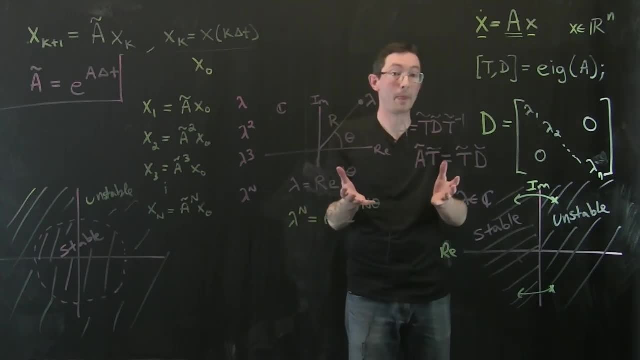 But the upshot, the thing I need you to understand and remember out of all of this, is that the stability of your system in continuous time or discrete time, completely depends on the eigenvalues of your matrix. In continuous time, you're going to be able to do this. 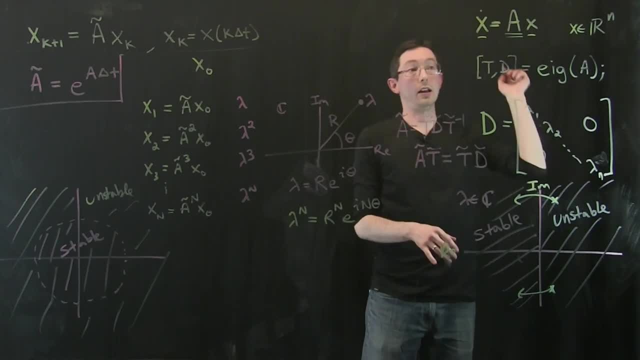 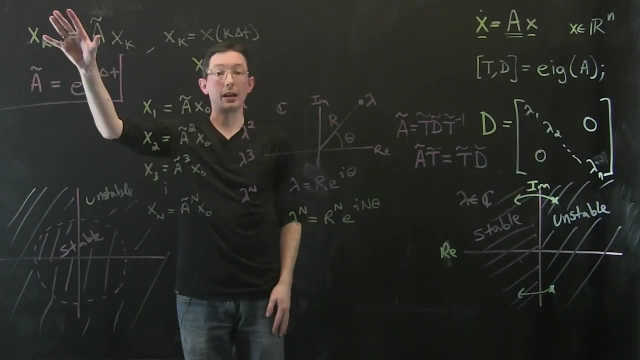 In discrete time. if the eigenvalues of your matrix have a negative real part, it's always stable. If a single one of these eigenvalues has a positive real part, it's unstable. And in discrete time. the analog is that all of my eigenvalues of a tilde